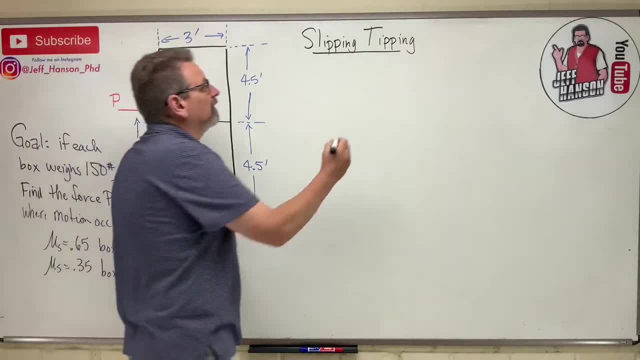 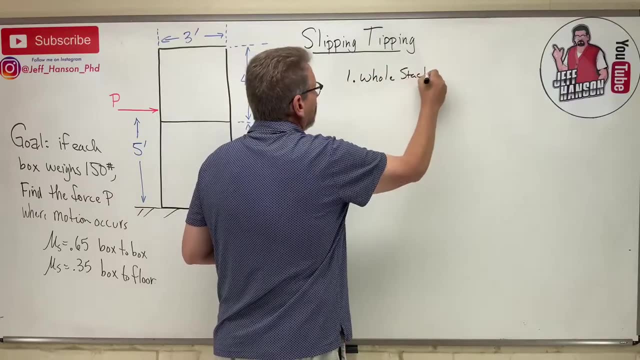 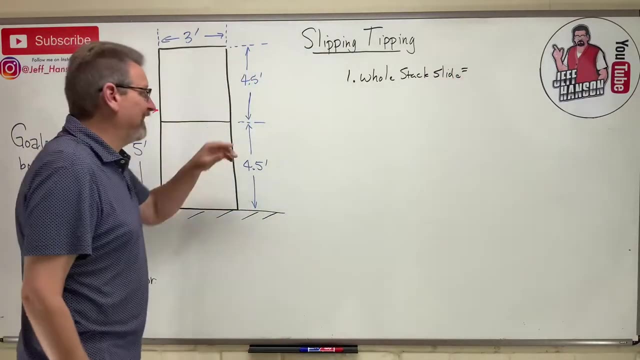 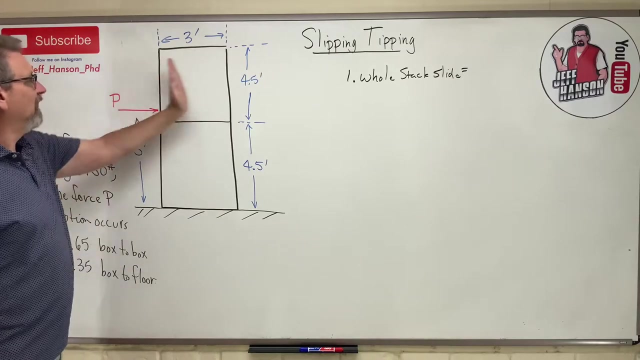 Well, okay, number one, number one: the whole stack can slide right. So I've got to find out the force P to make the whole stack slide. like the thing stays together and just slides right. What else can happen? Oh, the top box could just slide off and this box could stay. 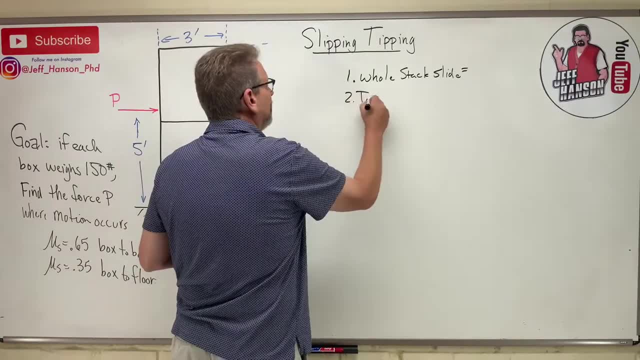 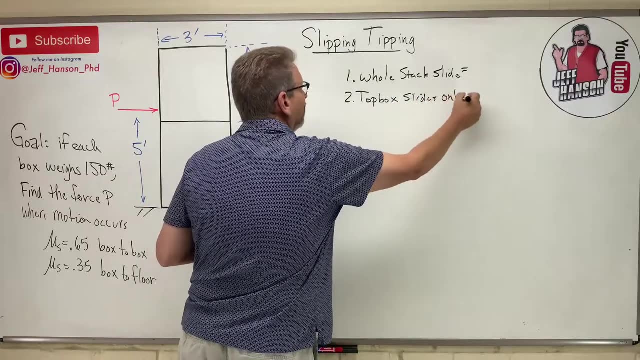 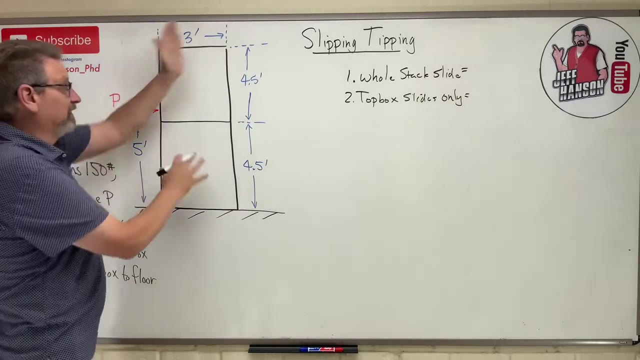 still okay. So number two, top box Slides, And I'll just put only right, It's the only one that slides, Anything else can happen. Well, I could push on it, What about it? The pile could just kind of like tip over. 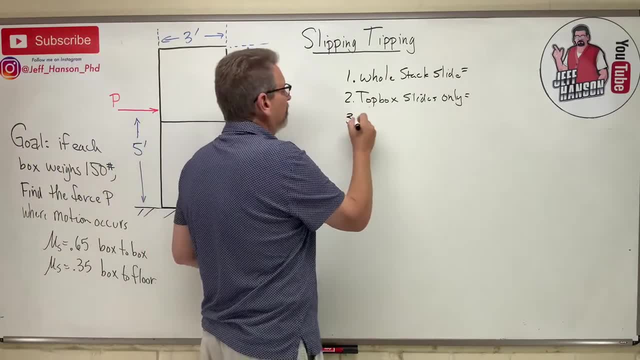 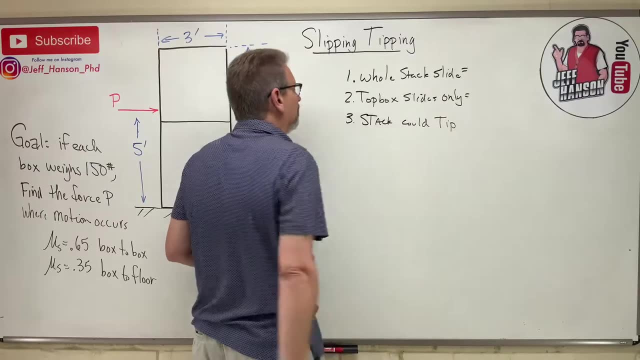 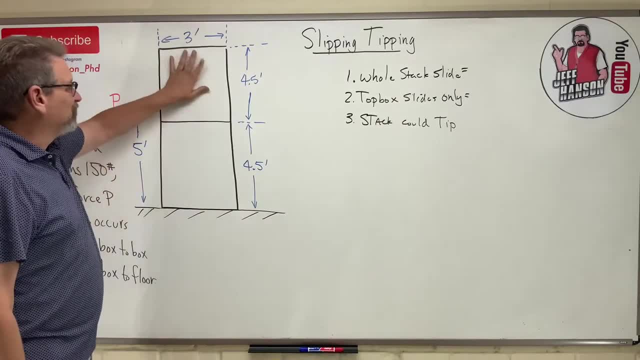 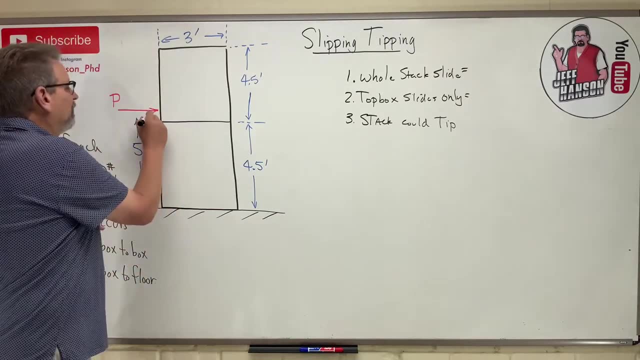 know, I don't know, I don't know, I don't know. Okay, This box can stay still and I could push on it and just the top box would tip. I don't think that could possibly happen because it's so close to the bottom down here. But you know what? Just for fun, we'll work it out and see. 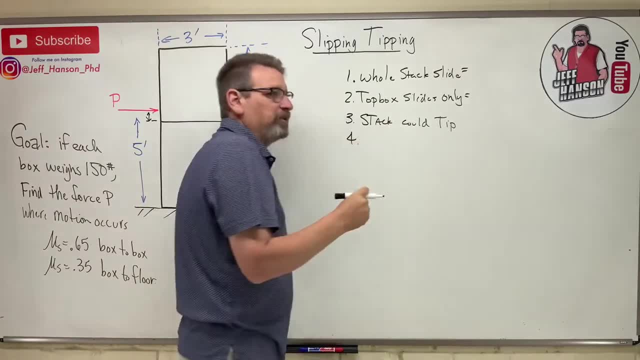 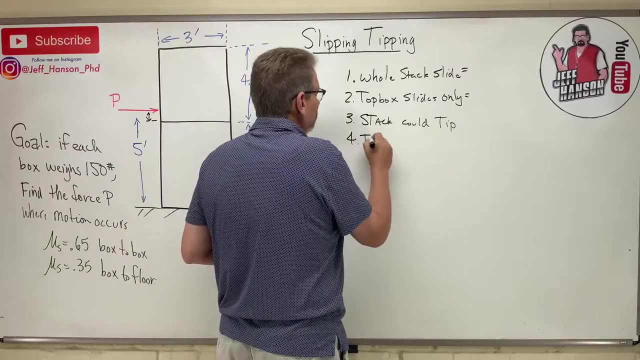 what it is, but I don't. there's like no way that would happen. That'd be like trying to tip your refrigerator by pushing on it. you know a foot off the floor, It's not going to tip over. You got to be up tall right, So top box tips Okay. So what we got to do is we're going to. 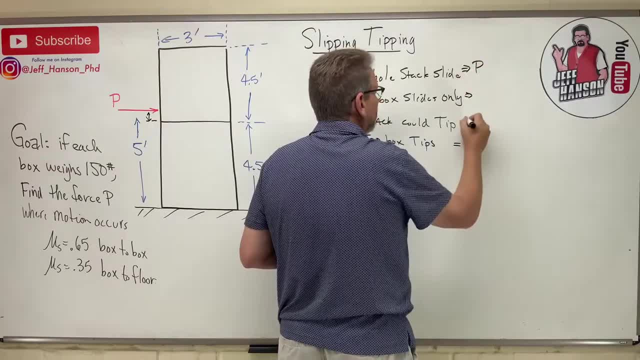 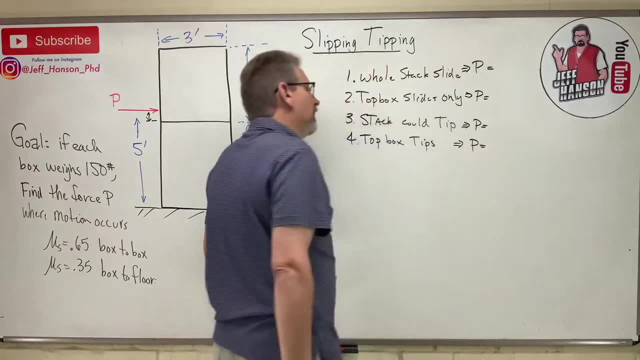 the goal here is to find a p for each one of these. okay, so we got to find p for that one. what is p for this guy, p for that guy and p for that guy? okay, and which one are we going to go for? we're going to have four different numbers over there. which one are we going to select for the? 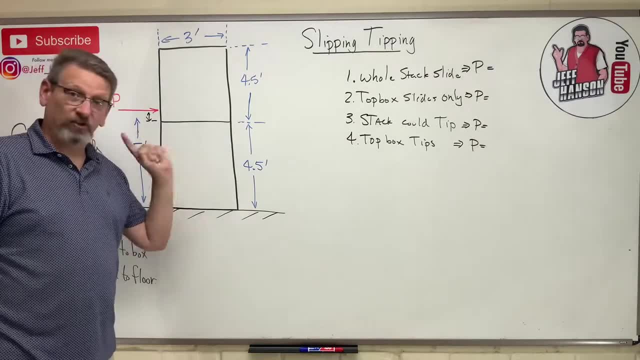 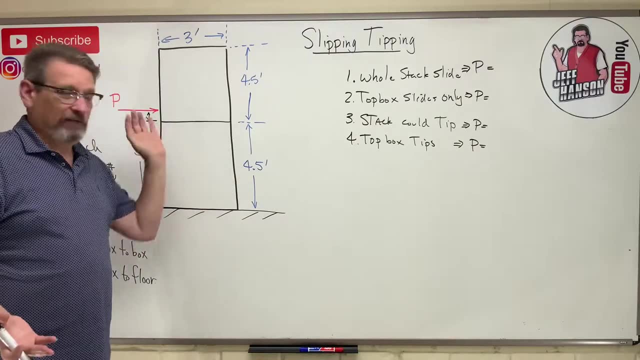 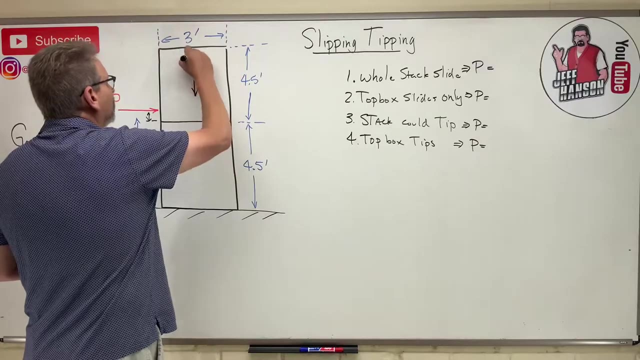 force p, where motion occurs, the smallest one, because that's the one that's going to happen first. right, you'll never get to those other conditions because that first motion happens first. okay, so let's- uh, let's- put our weights on here. just for funsies, there's a 150 pounds. 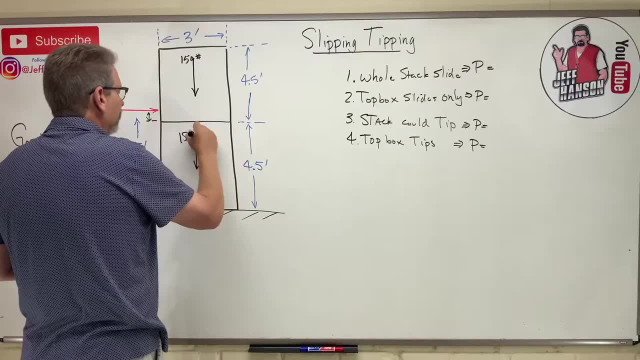 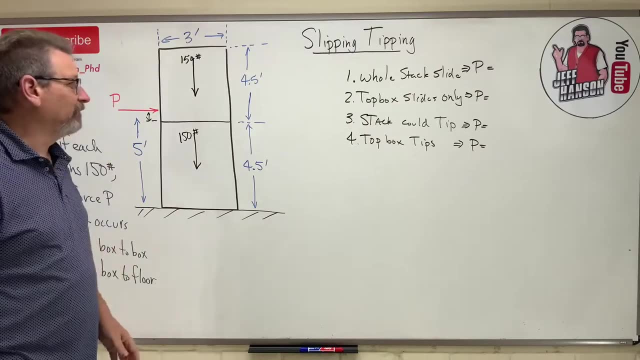 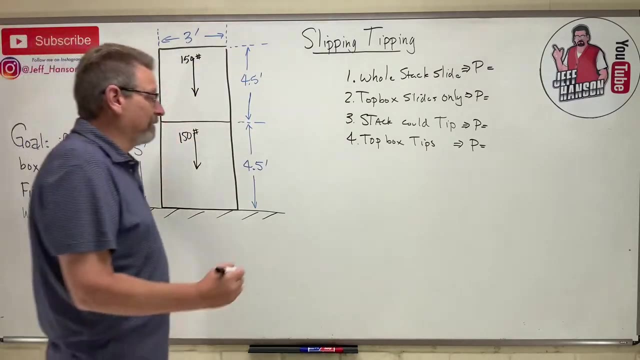 and there is 150 pounds. okay, so this solvent statics problems for friction is all, all, all about the free body. okay, so let's try the whole shack shimmies. i mean, the whole stack slides. okay, so look at this as one big box. okay, so here's one big box. 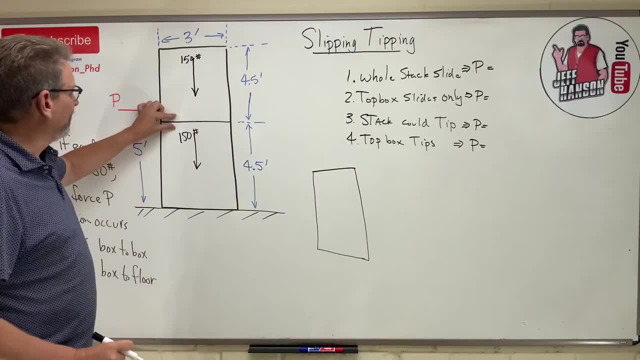 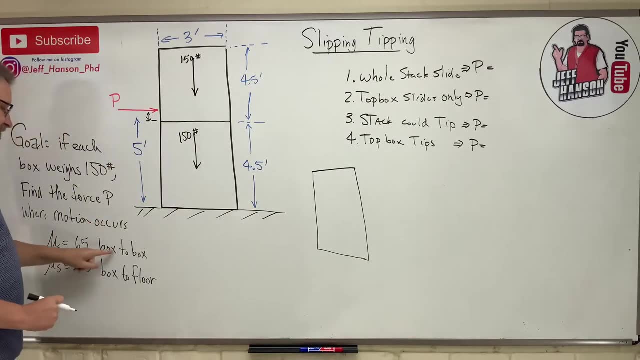 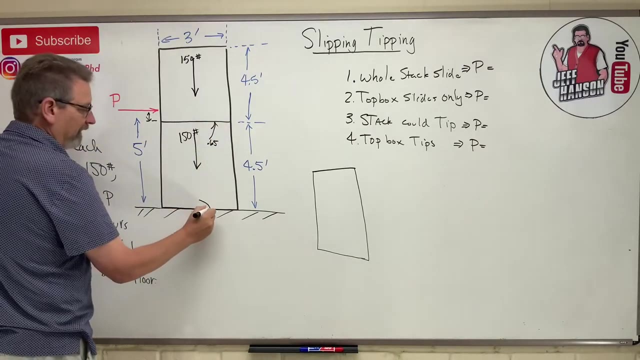 so what we're assuming for the whole stack to slide is there will be no sliding here. this is like very frictitious in there. right, this is so. this is like a look: box to box is 0.65 and box the floor is 0.35. 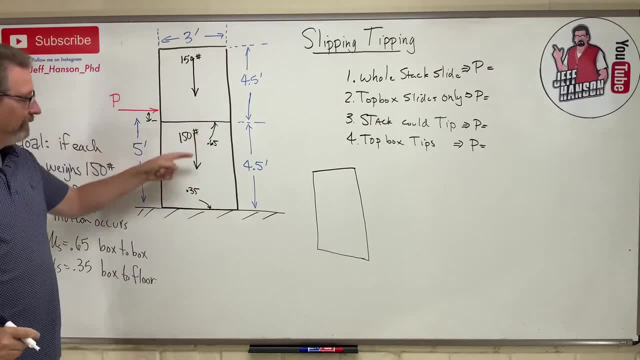 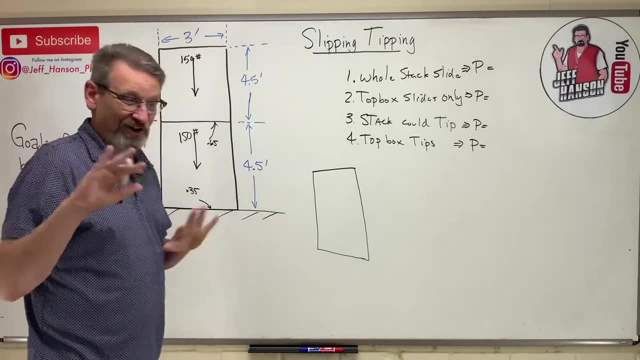 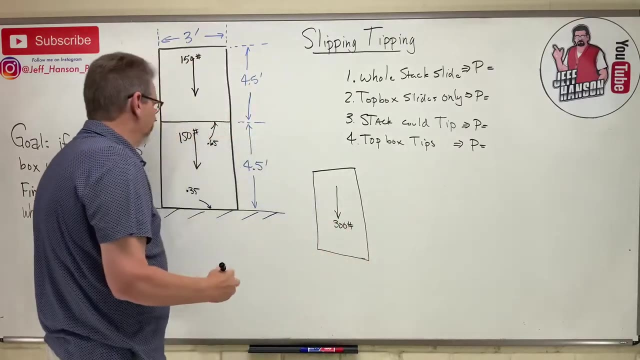 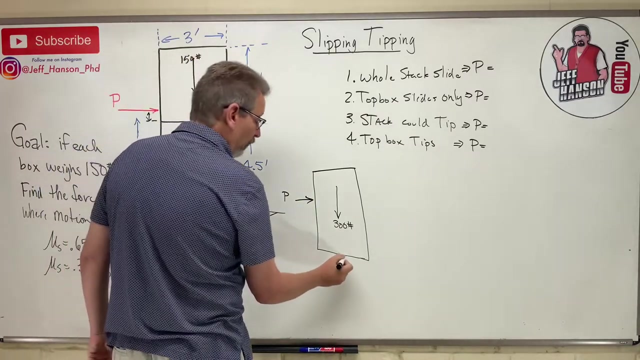 okay, so this is grippy and this is slippy, right, because it's got a lower coefficient of friction. okay, frictitious, not a word, but that's okay. okay, here we go. the box weighs 300 pounds. okay, because it's two boxes. here's our force p. okay, what else is going on? well, there's a normal force box. push on floor floor. 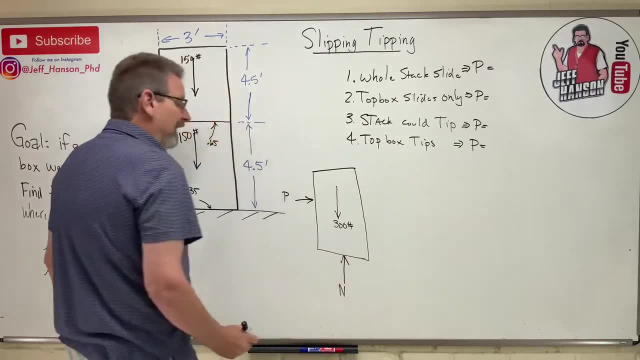 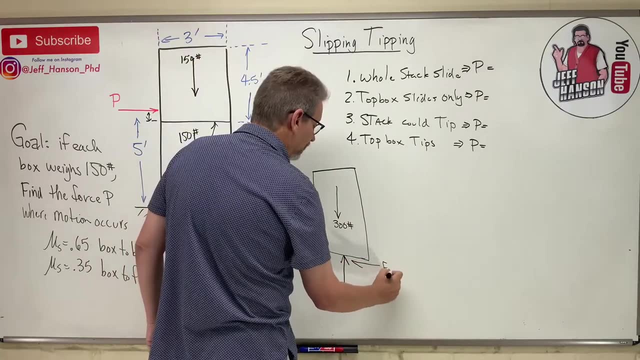 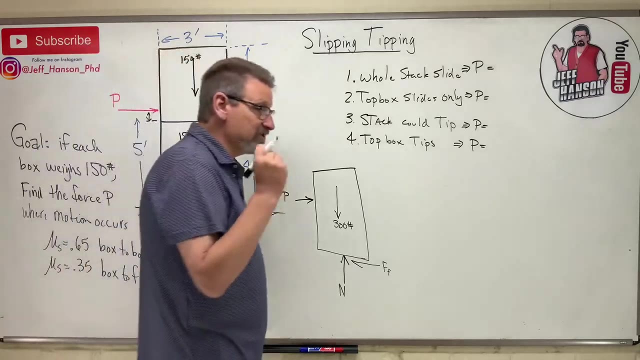 push on box, okay, like that, and then the box wants to slide that way, and so friction's like no, i don't think so, man. so friction, he's opposing us. he looks like that and we're looking about motion occurring, so we're at impending motion, so that friction down. there is fun friction. 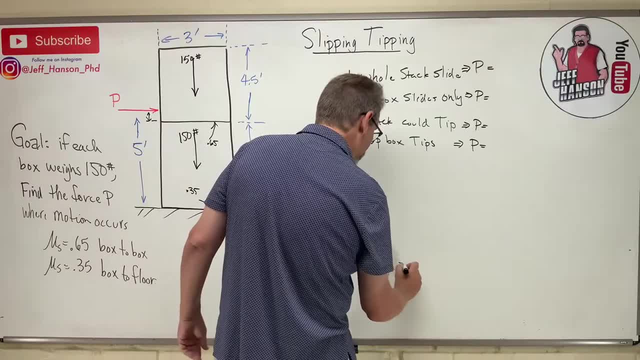 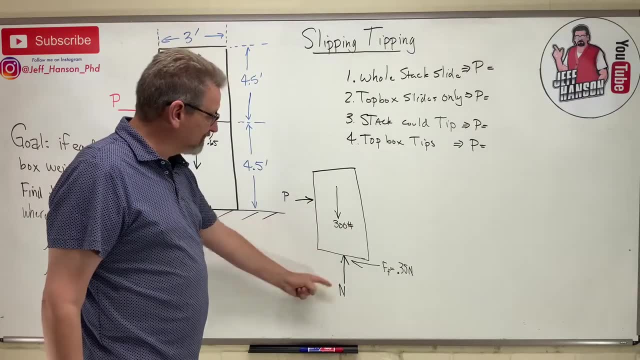 and the friction on the floor is 0.35. and there you go. so let's see what is the end going to be. some of the force in the y. i got 300 down. i got something going up. n has to be 300, doesn't it? 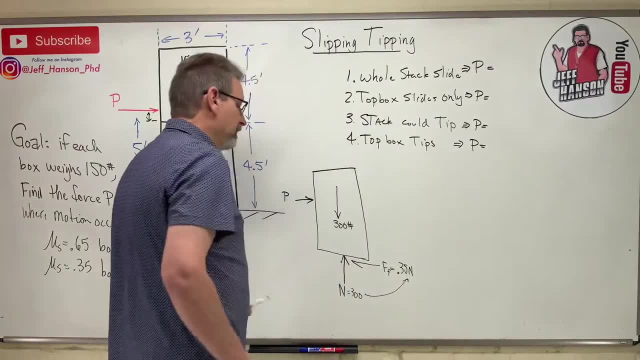 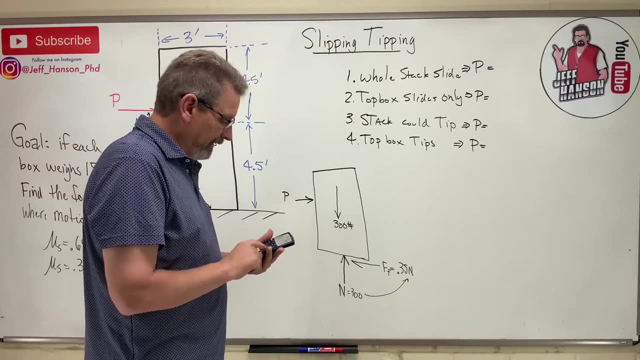 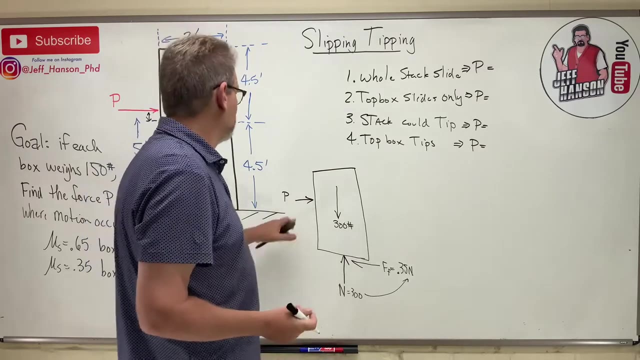 which we can plug whoop right in there, and friction force has got to be equal to p. so we're fixing to get p right here. right, p is equal to clear, clear, clear. 0.35 times 300 equals 105.. so p is 105 for the whole stack slides okay. 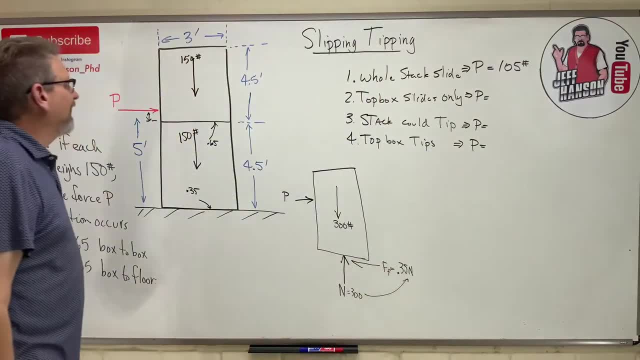 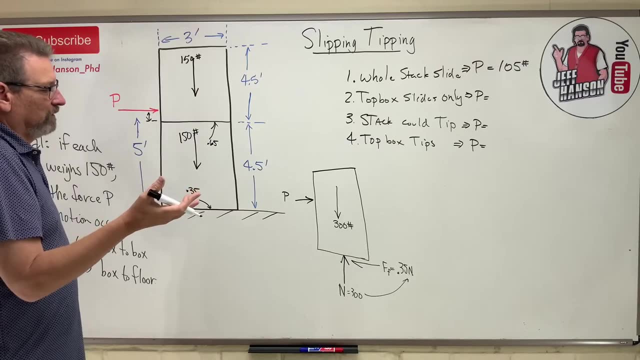 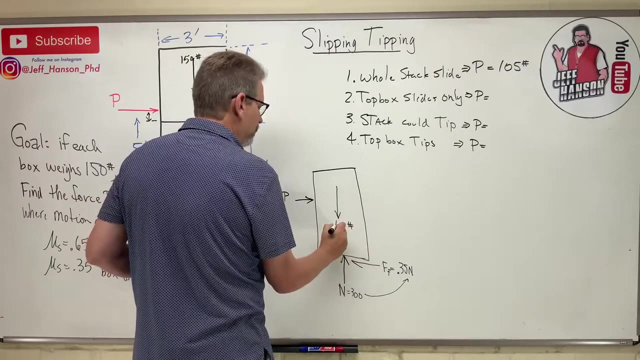 it takes 105 pounds to make that happen. okay, well, okay, fine. how about top box slides? only, okay, top box slides. so let me redraw my free body here. i'll get rid of this, because now we're just talking about one box. he's 150 pounds. um, what else do we know here? well, um, 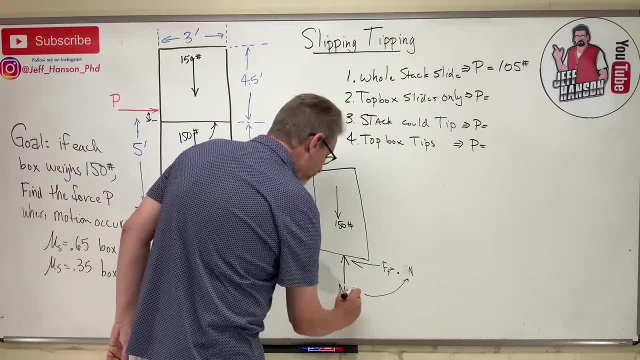 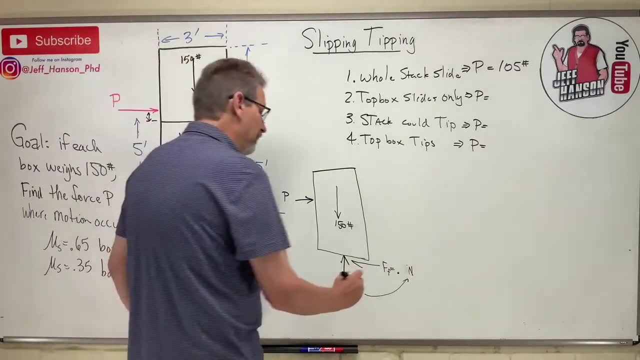 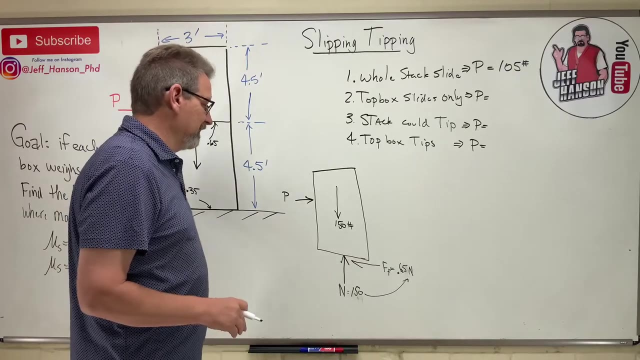 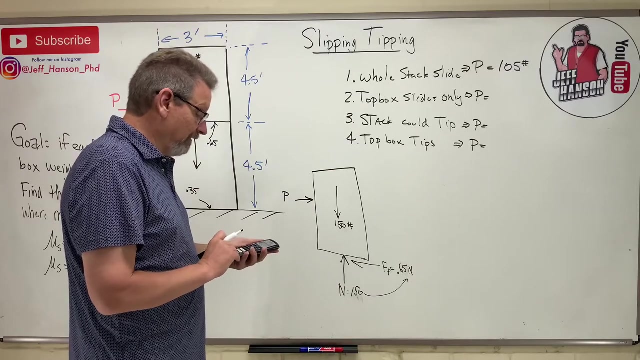 n now is going to be n is going to be 150 pounds. now, and let's see the static coefficient of friction. there is 0.65, so 0.65 and so p. now for just the top box to slide is how much is that? okay, 150 times 0.65 equals 97.5 statics radio tune in now. 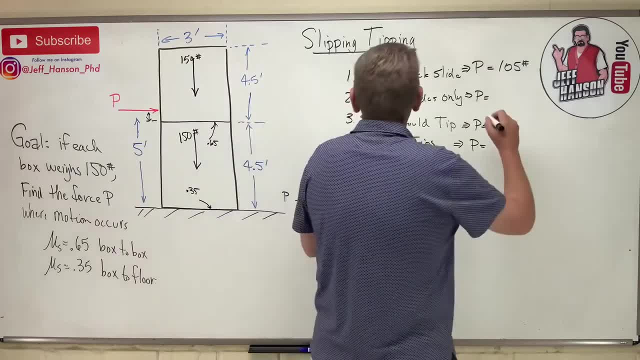 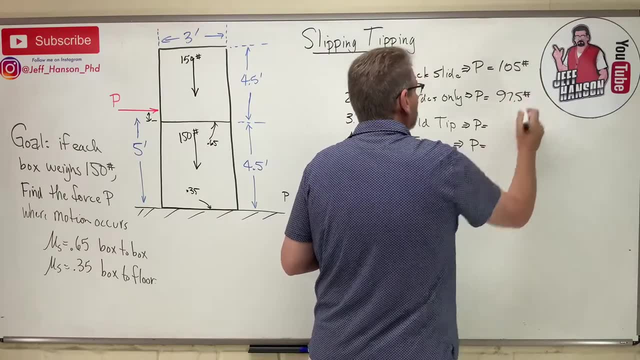 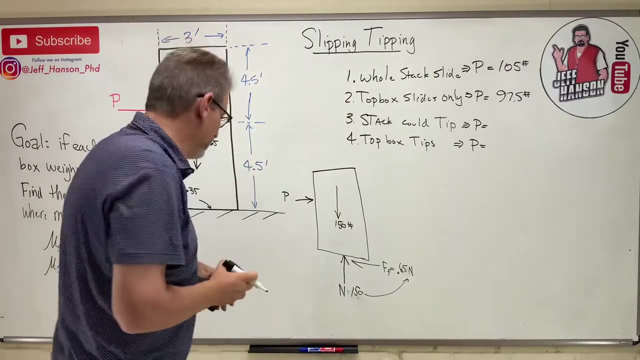 and we'll get frictitious up in here. okay, 97.5, where? what? that's top box, 97.5 pounds. okay, well, the whole stack is not going to slide now. this guy's winning right. the top box slide is going to be 0.65. so that's the top box slide. okay, let's see what else we got. okay, next is: 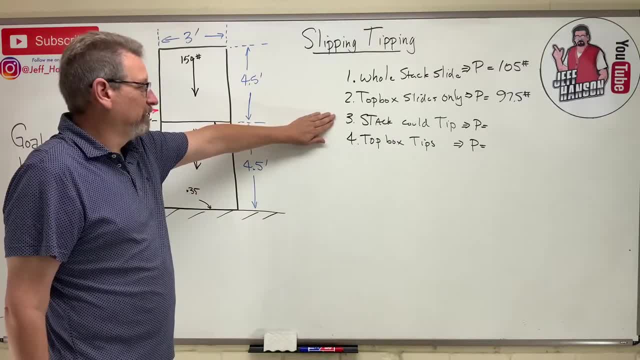 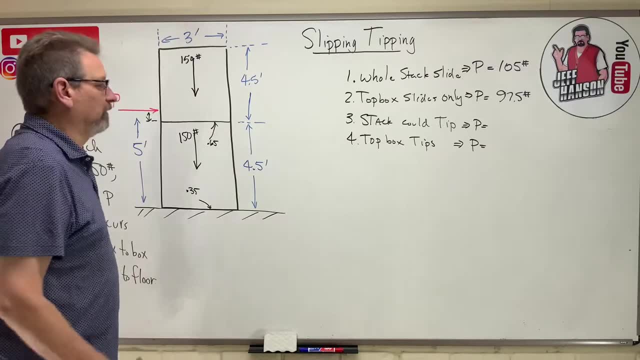 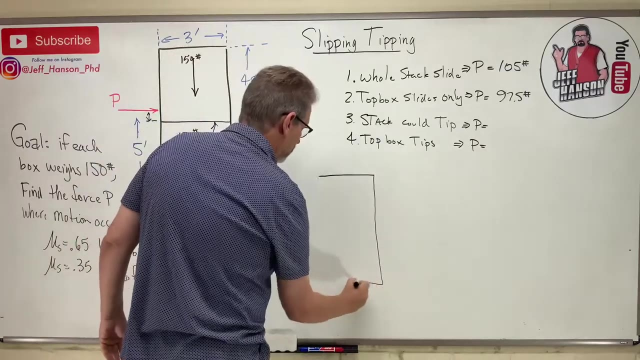 number three: the stack could tip okay. so if this pile of boxes here starts to tip, right, where is it going to rotate about? well, it's going to rotate about this corner, right there, isn't it? so let's do this. let's draw a box. we're back to the big box again. okay, i'm going to call him 300 pounds, okay. 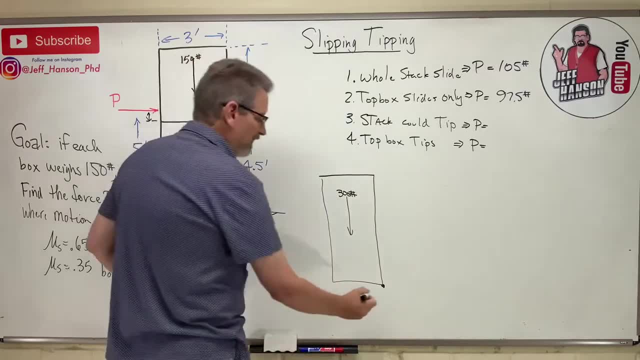 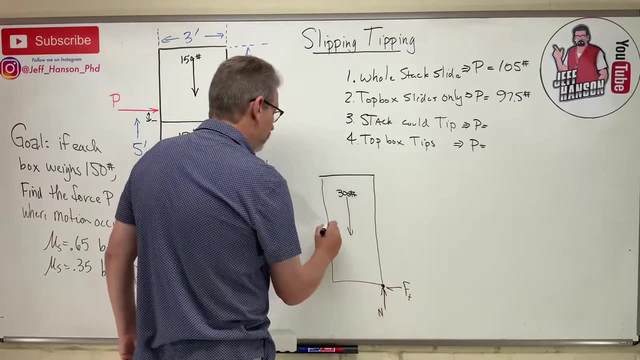 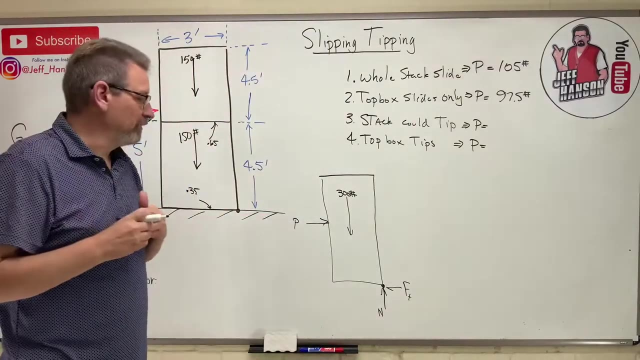 and it's going to tip about that corner right there, right? so you've got like a normal force there and a friction force there, and then here's force P over here. okay, whenever you have tipping, you need to think moment equation, don't you? okay for the moment equation? all right, I'm gonna take the moment at this corner. 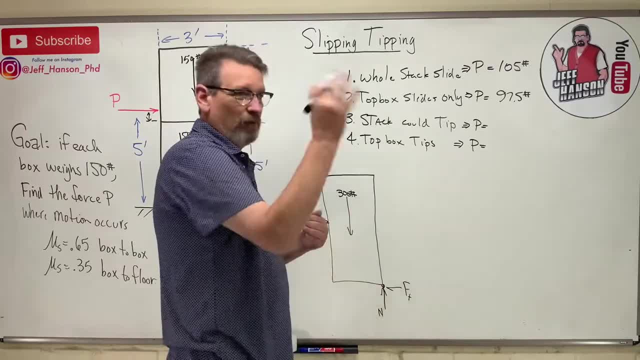 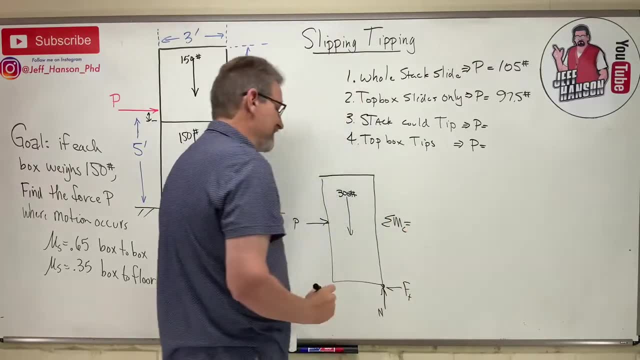 because it's trying to rotate, okay. so think about tipping rotate moment, rotate, okay, that goes together. so here we go. let's sum the moment about. I'll call it point C for the corner. C is for corner, and what do I have? I have the 300, which. 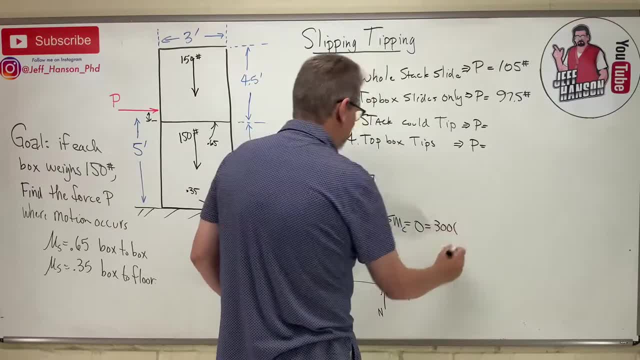 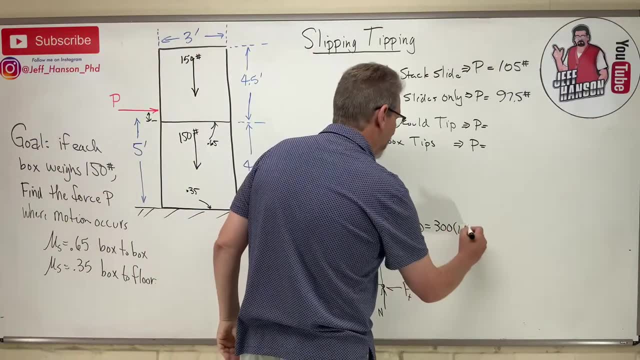 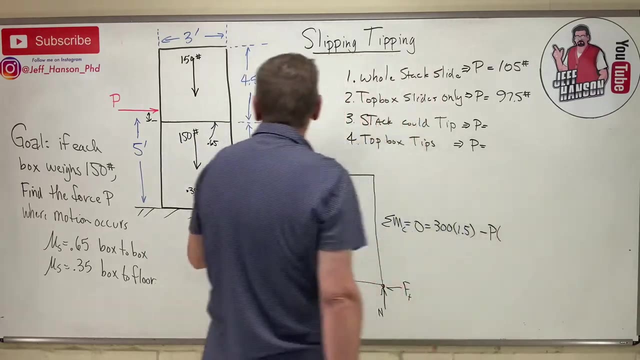 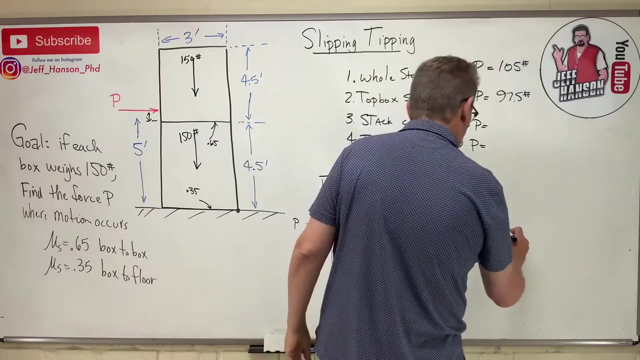 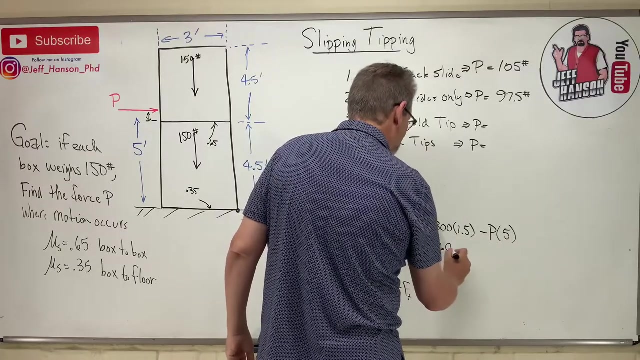 rotates me positive, so 300 times. how far away is that? right, it's a one point five, isn't it one point five? and then the P rotates me. oh, that's negative minus P times. how far away is that? it's five, isn't it okay? so that's 450 divided by five. P is equal to 90 pounds. 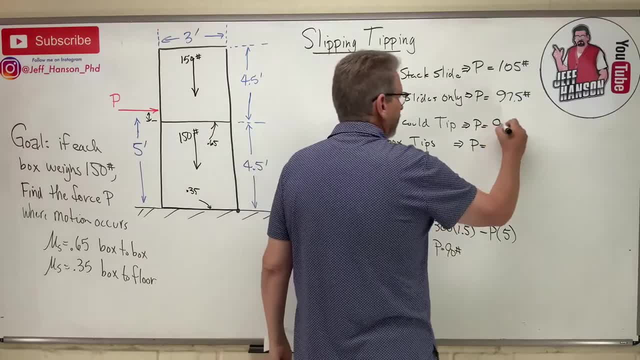 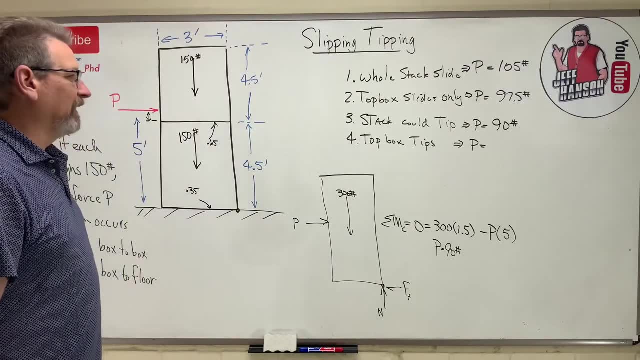 oh, we've got a new winner, don't we? it only takes 90 pounds of force to make that stack start to tip over, okay, and then we can talk about: let's do, let's do crazy town here, because somebody will get me in the comments on this if they. 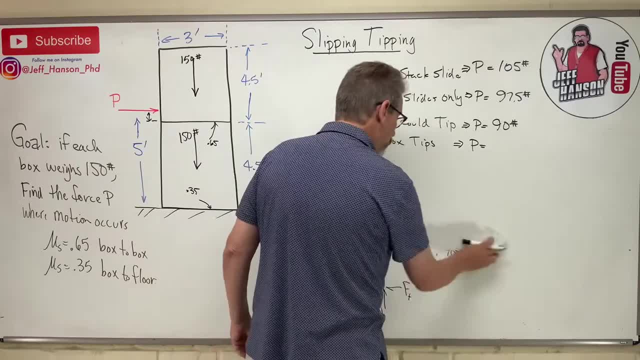 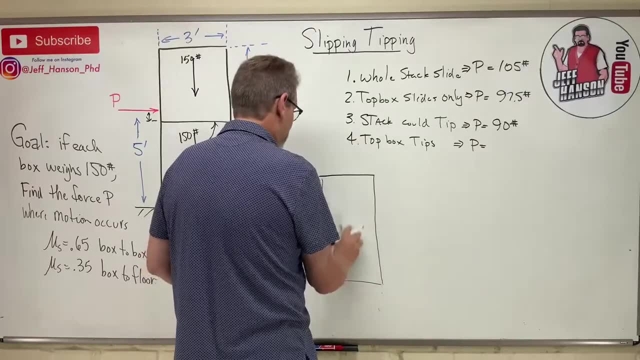 don't, if I don't check it, they'll be like: but you should have worked that other one. it could have happened- yeah, it could have- if this corner was like glued together and then it would have worked. but it wouldn't have worked if it was together. I don't think it's gonna happen, but let's just try it, okay. so now. 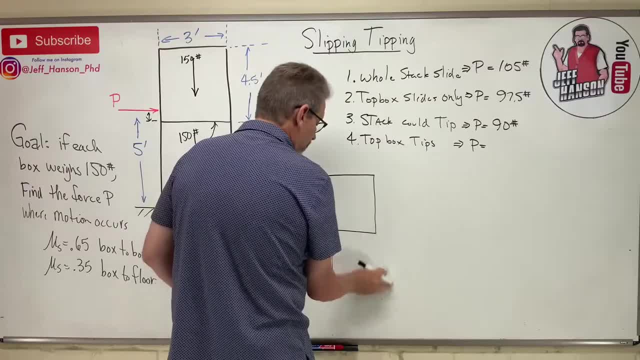 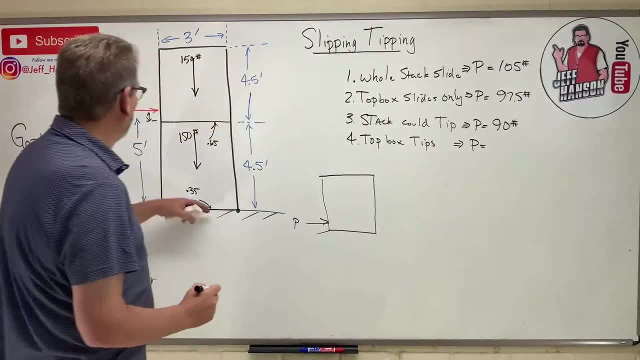 the box is only like that big. okay, so now we're talking about just the bottom box. stay still, and only the top box tips, because this little distance here is what it's. four point five. it's only, it's only a half a foot right, point five. 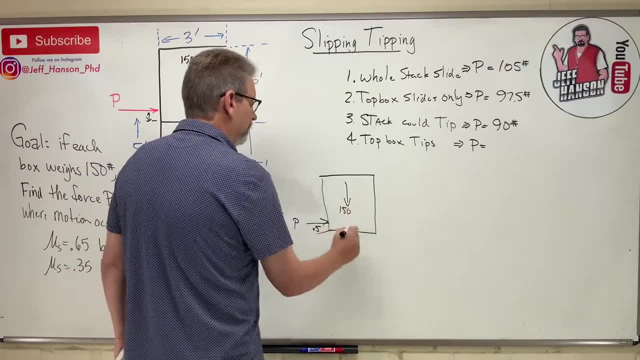 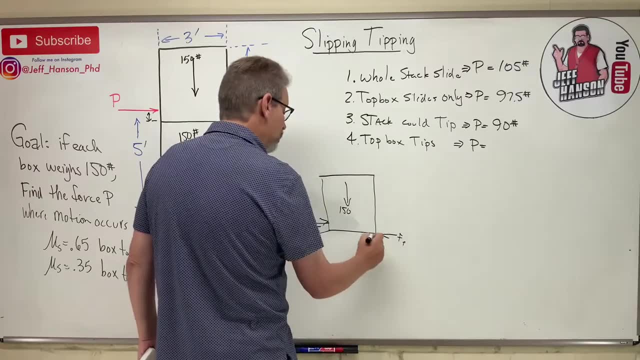 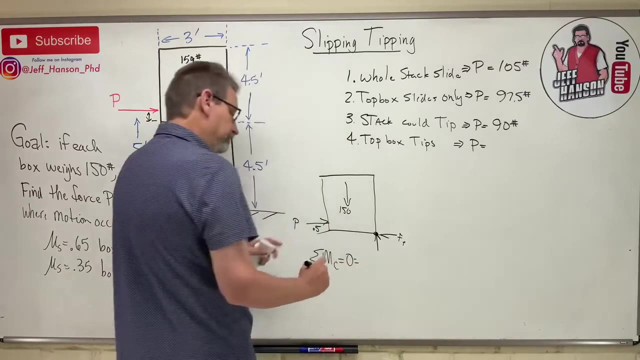 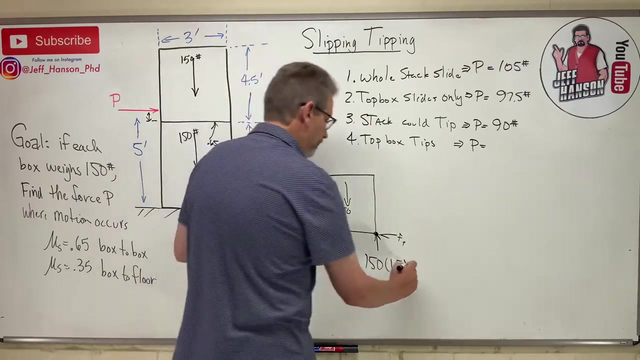 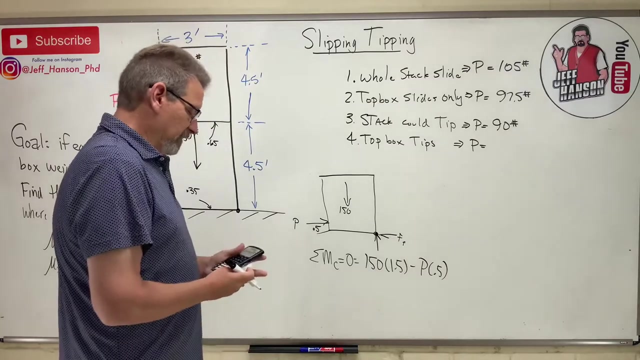 here's the 150. okay, that's gonna have to be like super glued down for this to stay over here, right, okay, so I'm gonna take that moment about that corner again. moment about the corner is equal to zero, is equal to 150 times 1.5 minus P times 0.5. oh goodness, okay, that's gonna be a. 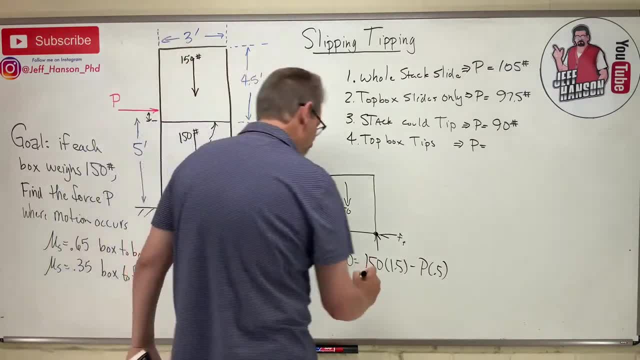 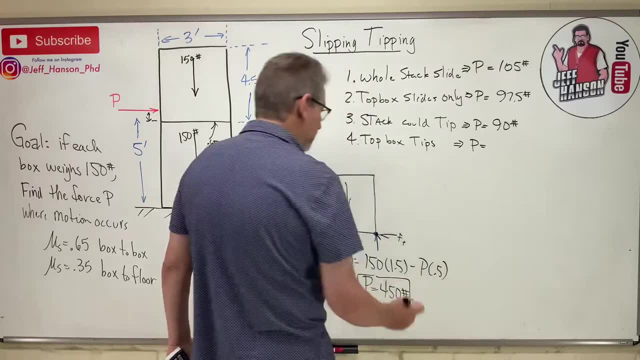 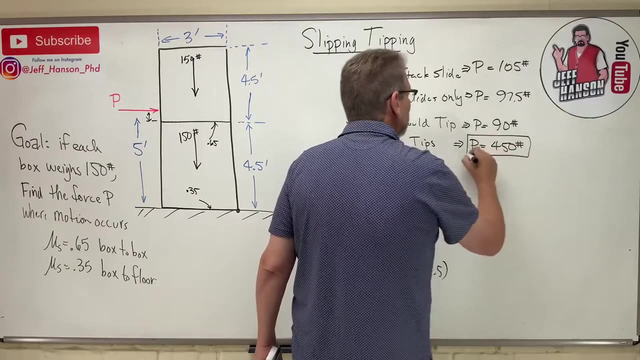 that's 450, isn't it? I can I do the math in my head: P is equal to 450 pounds. okay, so ain't no way that's happening. okay, 450 pounds, that's never, ever gonna happen, is it? so the thing I like about this problem is is you've got to come up with 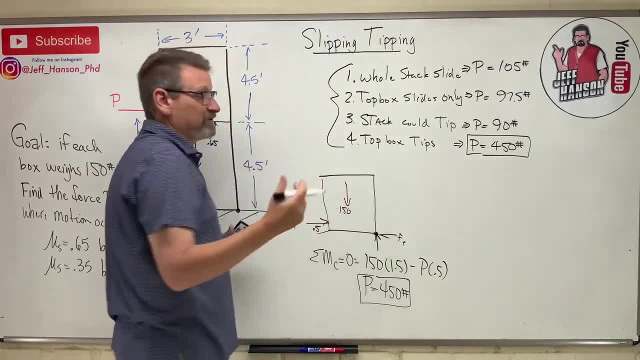 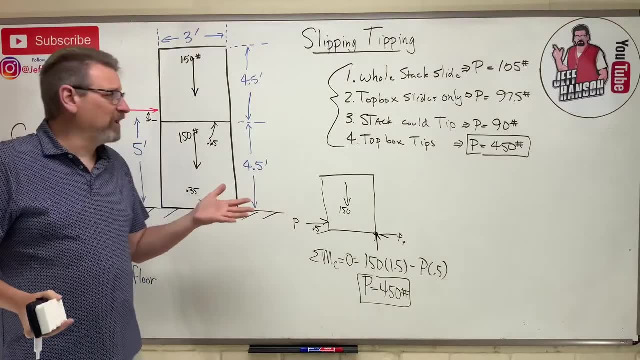 these scenarios right here on your own. when it says is motion can occur, you've got to think yourself: okay, what does that mean motion? can it slip? can it tip right? so you got to go through all those scenarios. okay, there's lots of problems like these. I really like these for a 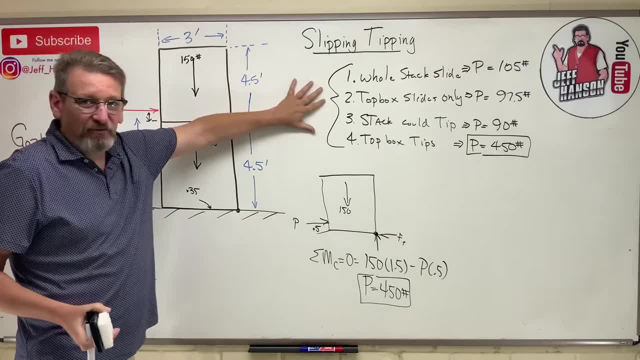 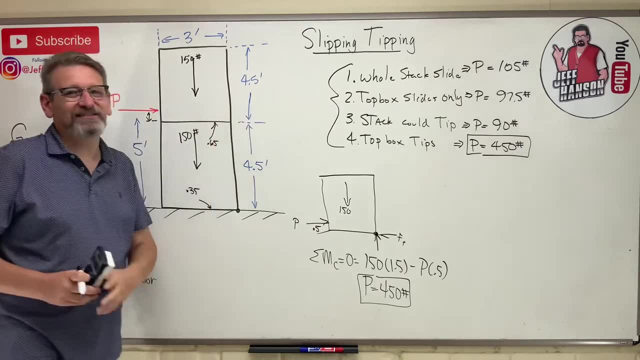 test, because this tells me the people that can think versus the people that are just trying to memorize equations. so can you think? I hope so. all right, I hope this helps and I'll see you back here next time, gang.